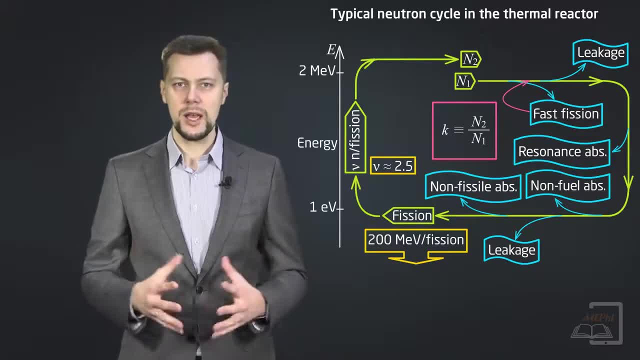 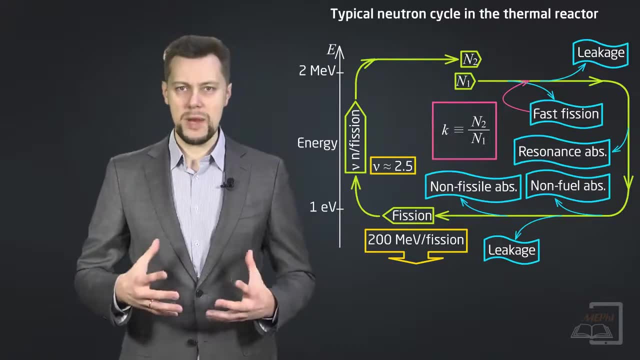 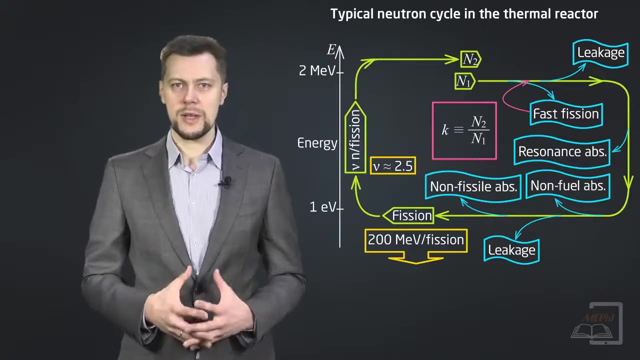 absorbing in, for example, non-fuel absorbent or in a fuel but not acyl, reaction occurs. It's bad too, And finally they can produce the fission. We get two hundreds megaelectron volts, energy Release N2 or three additional neutrons for. 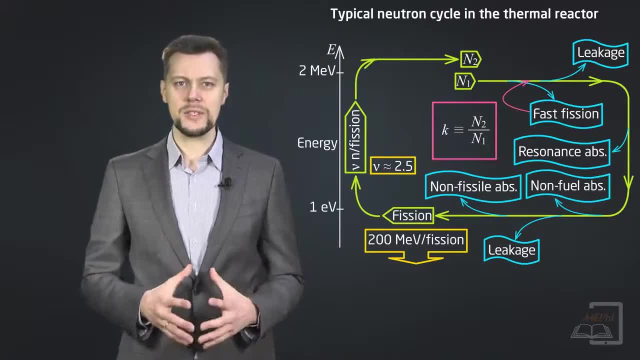 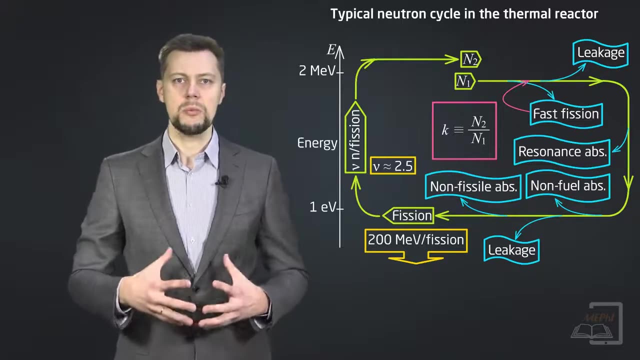 chain reaction. Let the number of neutrons after a whole cycle is N2.. N1 and N2 previous and following generation of neutrons. Thus K equals the ratio. N2N1 is the multiplication factor of the system reactor, which takes into consideration all Newton process. 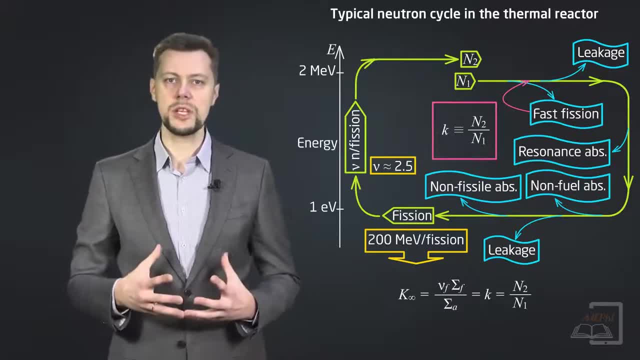 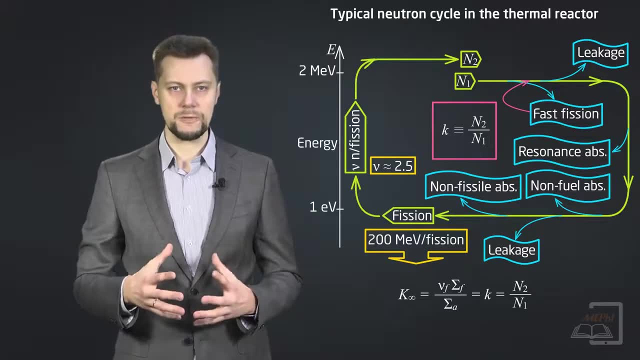 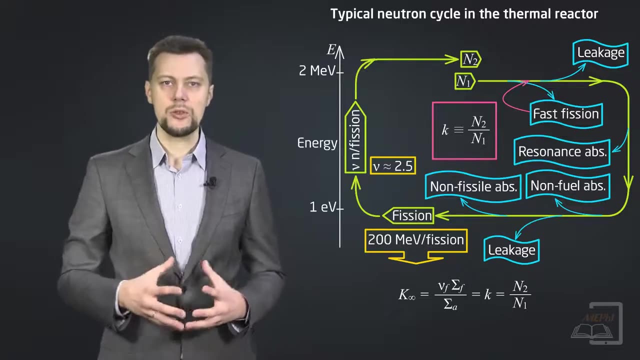 For infinite homogeneous medium. the definition of multiplication factor is the same to the factor of μF, σF and absorption: macroscopic cross-section. Please note that to slow down or not, it's our decision. it's our choice of reactor core design. 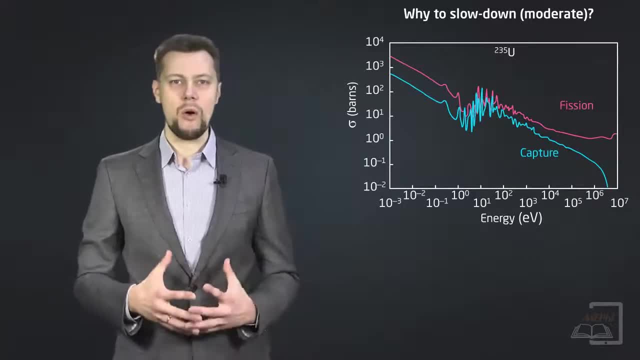 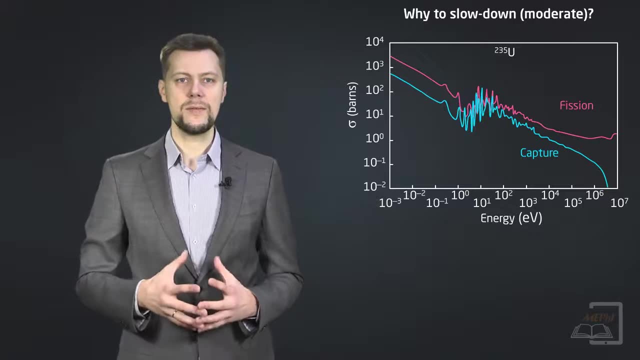 The reason of slowing down lays in the dependency of microscopic cross-section of fission. You can see that in fast energy range σF equals about several barns, but in thermal range σF equals hundreds barns. That means in thermal range the probability to make fission is much likely compared to fast range. 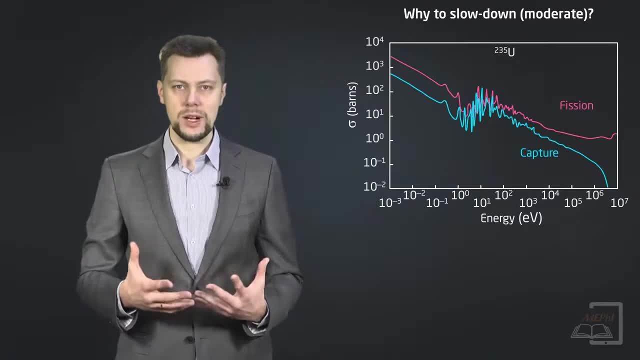 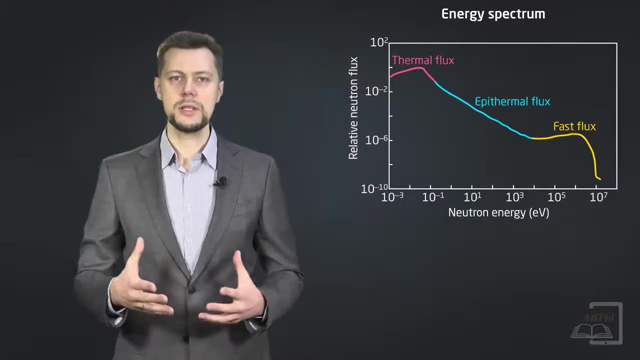 In turn, we need less uranium fuel for thermal reactors. They are more simple and cheaper as fast reactor. This part we should consider: the main laws of Newton slowing down process, And the second discover the dependency of Newton flux by energy. The last one is called Newton spectrum. 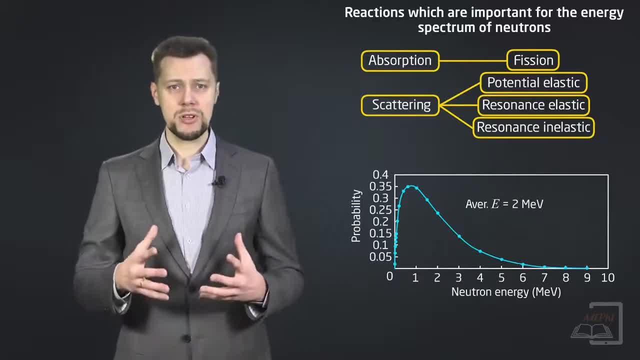 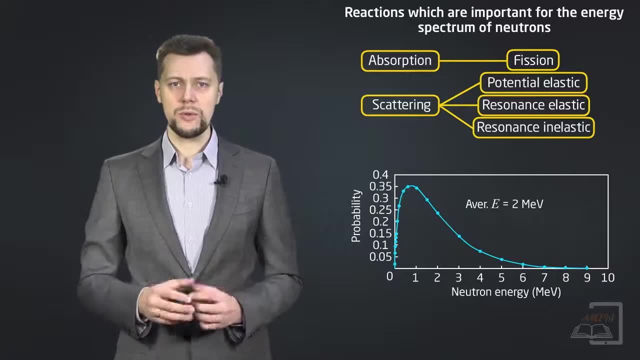 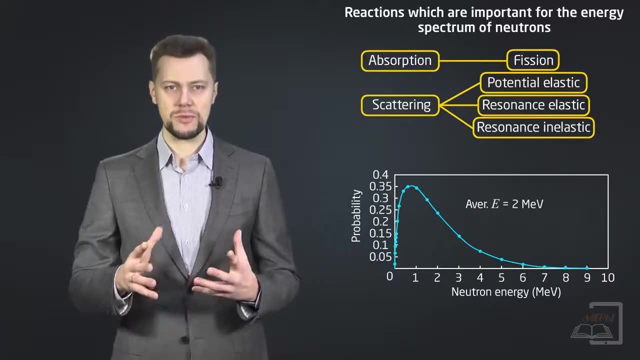 How can we slow down the neutrons? Of course, by nuclear reaction, of interaction of neutrons with nuclear of medium. We know two types of nuclear reaction: absorption and scattering. All these types have the influence on Newton spectrum. The absorption reaction influence means that after fission, 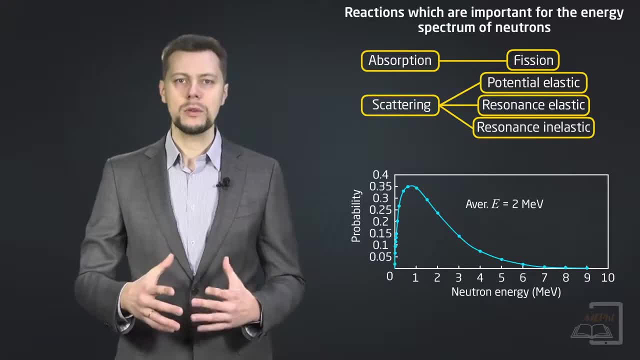 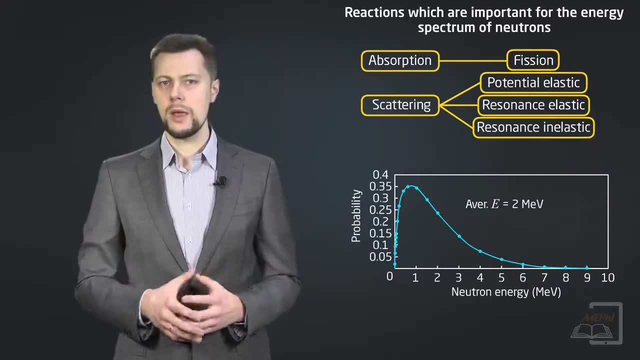 the fast neutrons have certain energy distribution called fission spectrum. The average Neutron energy is about 2 MeV. The main process of slowing down is scattering. The resonance in elastic scattering can moderate the neutrons. It's important but it's not the main process. 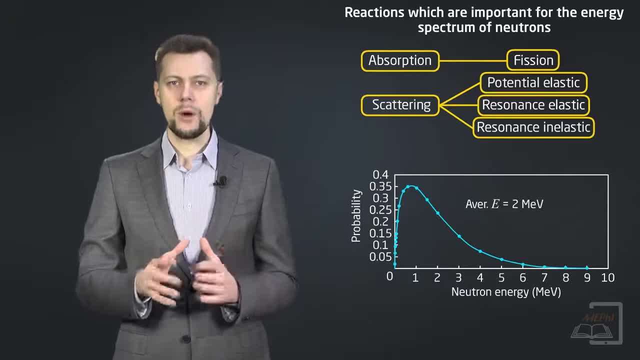 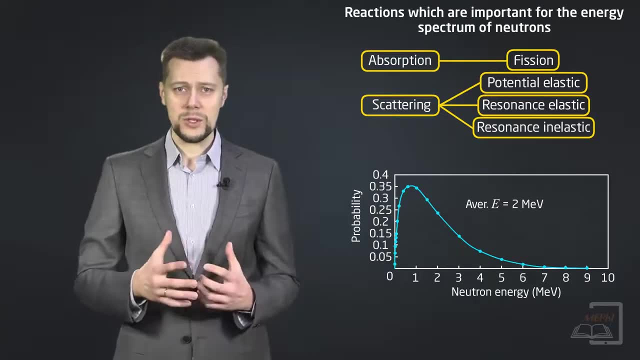 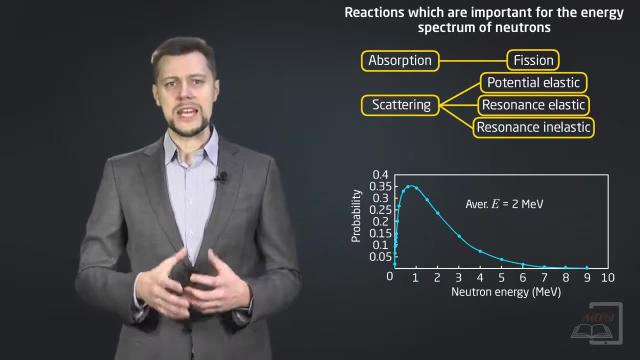 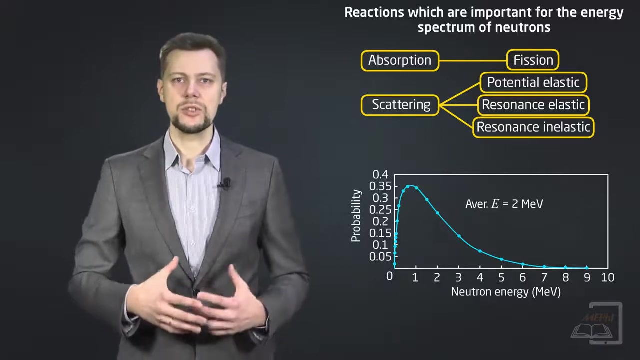 Because resonance levels for light nuclear are in fast energy range and for heavy nuclear the lowest energy level is in the range of kilovolts. It's not enough. The resonance elastic scattering does not moderate neutrons, So the main nuclear reaction to neutron slowdown is potential elastic scattering. 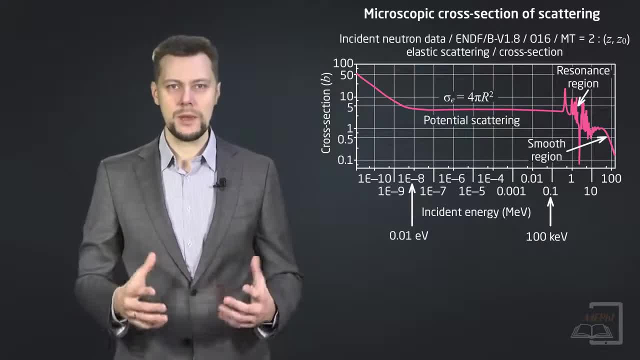 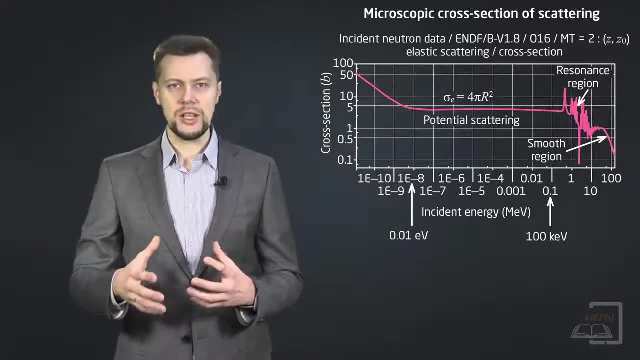 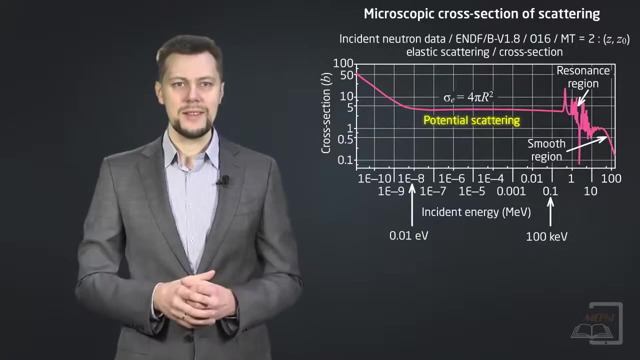 Look at the typical microscopic cross-section of elastic scattering. As usual, there are three region-independency microscopic cross-section scattering to energy in epithermal energy range. The first is table-length zone. This is potential elastic scattering. The second is resonance zone. 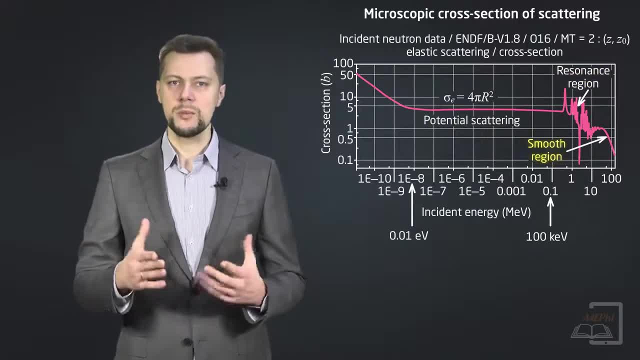 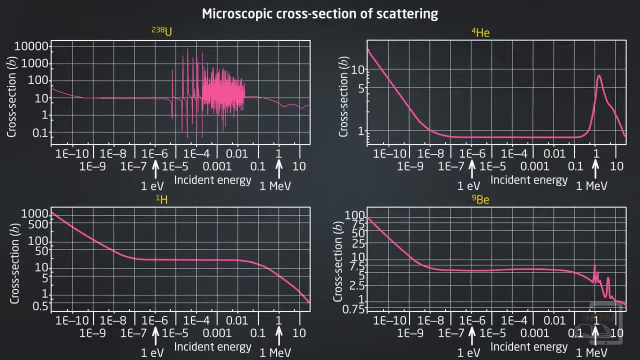 This is resonance elastic scattering, Smooth region. Too many resonances form the smooth region, So the potential elastic scattering is table-length zone-independency elastic scattering. This is the main reason for the smooth region. It is limited from the right by the resonance zone. 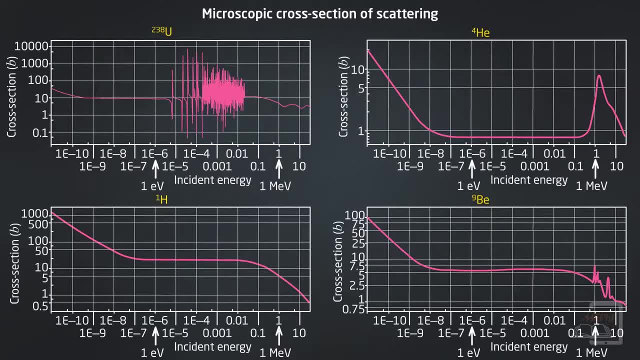 Excluded hydrogen and deuterium. For light nuclear the potential elastic scattering takes place till hundreds of kiloelectron volts, In contrast to heavy nuclear, for example uranium-238,. the right border is in the range of electron volts We can define the slowing down energy range. 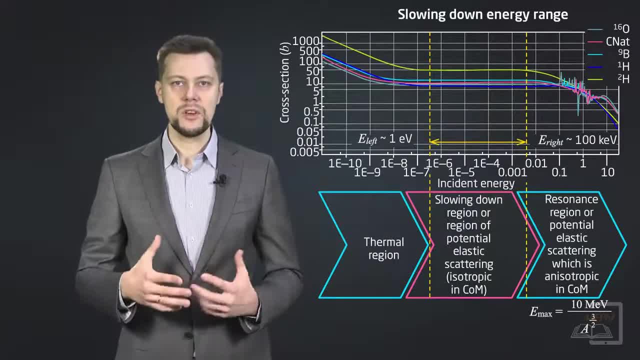 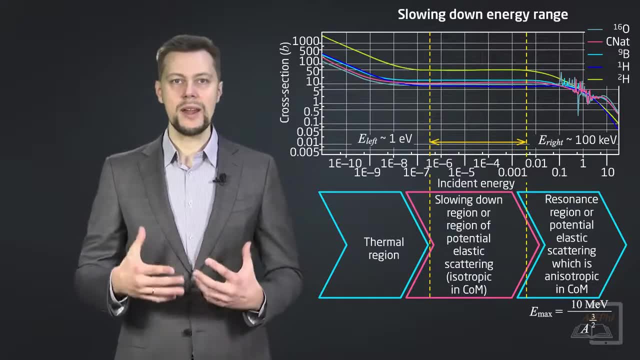 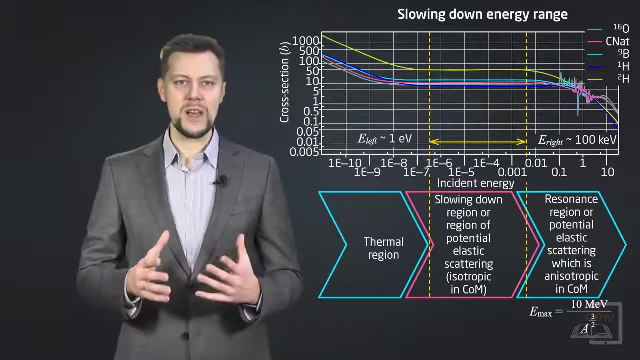 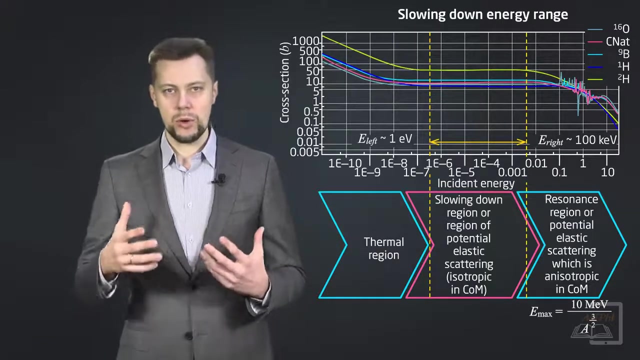 The following development of laws, formulas and equations will be true for the region. It will be our main approximation. The slowing down range is limited from the left by the thermal range about 1 electron volts From the right, the first by the border of potential elastic scattering and the second